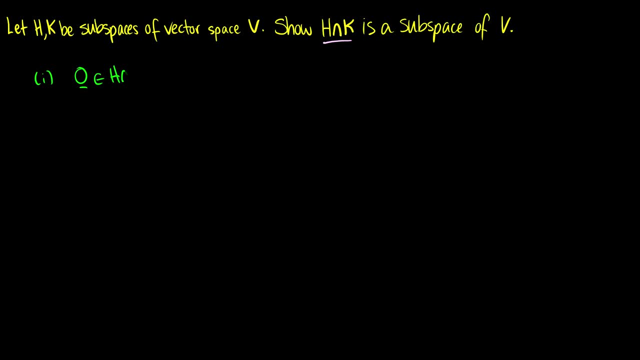 is, we have to show that the zero vector is going to be an h, intersection k. So well, h and k are subspaces. so that means that the zero vector is going to be an h and the zero vector is going to be in k. therefore, the zero vector is going to be in the intersection, since 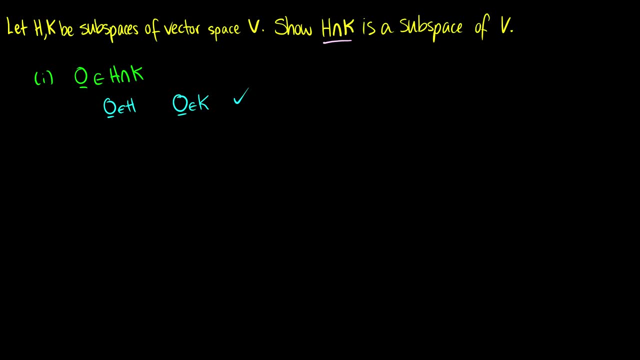 it's going to be in the intersection, If you may have forgotten the intersection. so if I say x intersection y, this is the set of all x, such that x is in big X and x is in big Y. So that is the intersection. It's going to be in both. Okay, so the zero vector is in both. therefore it's in the. 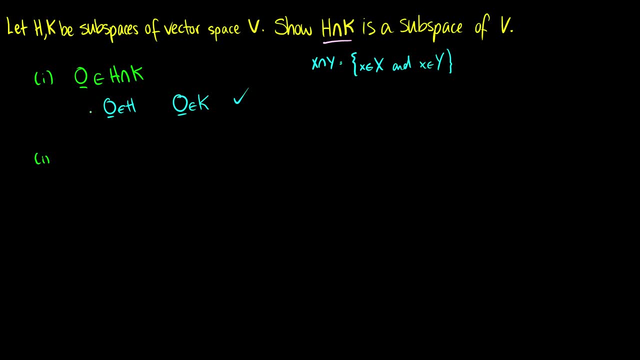 intersection For two. we want to show that if we have- so let's say we have u and v in h intersection k- then we're going to have u plus v in h intersection k. So let's suppose we have vectors u and v in h intersection k. So then what we know? 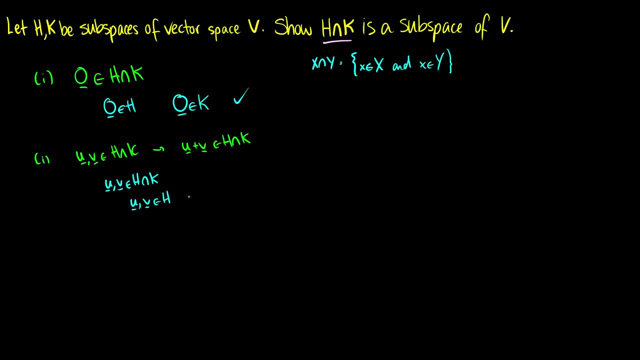 is we know that u and v are going to be in h and the vectors u and v are going to be in k, Since, by definition, if they're in the intersection they're going to be in both, And because h and k are subspaces, if u is in h and v is in h, then we know that u plus v is going to be. 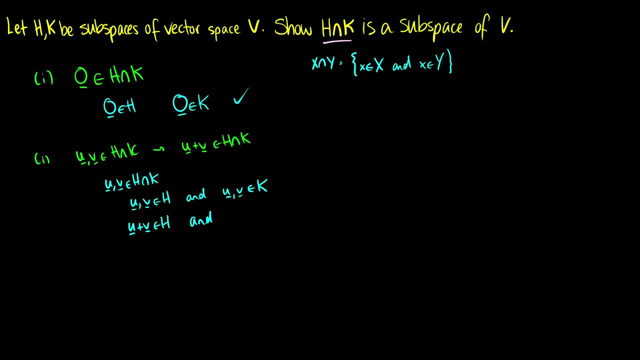 in h, and if u and v are in k, then u plus v are going to be in k. Therefore, u plus v is in h and u plus v is in k. so we're going to get: u plus v is in the intersection of h and k. That's condition. 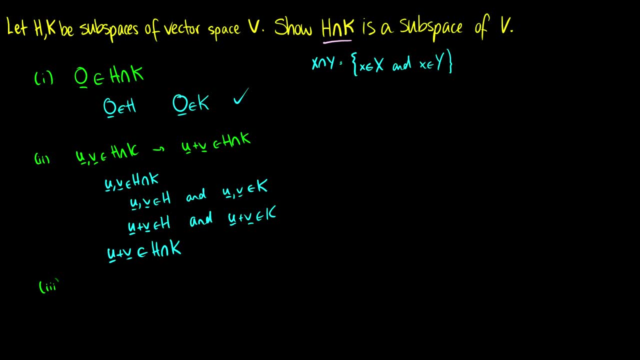 okay. So condition number three says that if we have, say, some vector u in h intersection k, then we're also going to have any scalar c times u in h intersection k. Well, first thing we're going to do is we're going to assume we have this u in h intersection k. so 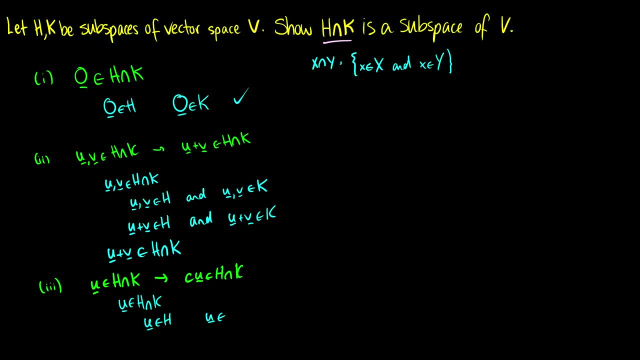 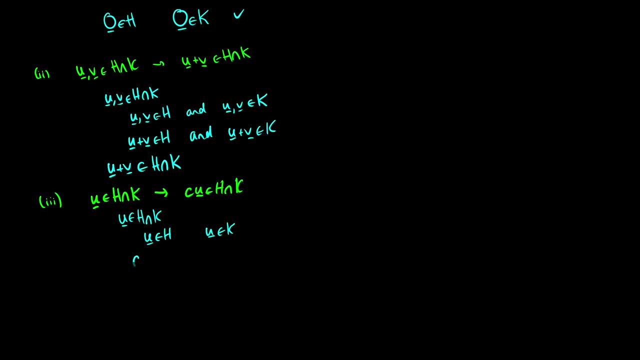 this means that u is going to be in h and u is going to be in k, because if it's in the intersection, it's going to be in both, and because h is a subspace, any scalar times, u is going to be in h. because k is a subspace, any scalar times u is going to be in k. any scalar times u is in both of these. 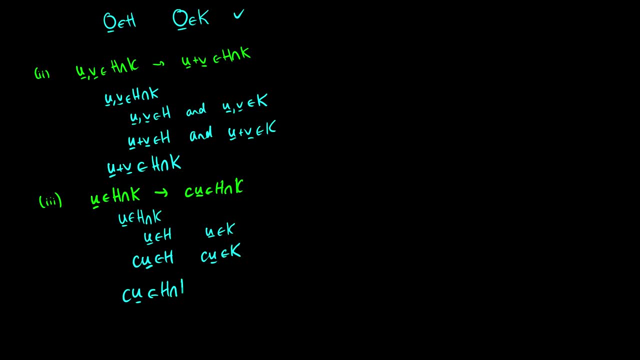 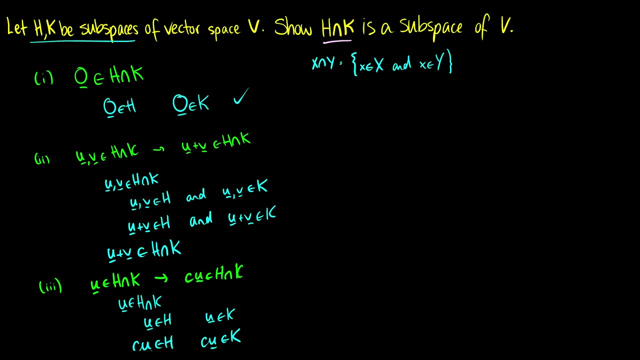 therefore c times u is going to be in the intersection of h and k. So therefore we have proven that if h and k are subspaces, then h intersection k is also going to be a subspace. Okay, so that's the first proof. Second proof, a little bit easier: suppose we have a scalar times u is equal to the zero vector for 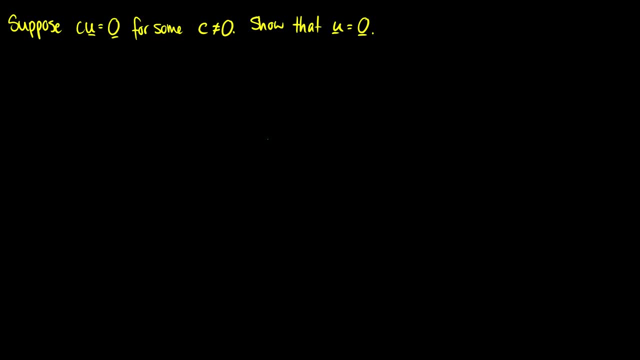 some non-zero scalar. we need to show that u is equal to the zero vector. I know this. this seems really intuitive. so if I have, like three times the vector, u is equal to zero. obviously u is going to be zero, but let's prove that. So let's start with u. we should start with one times u. 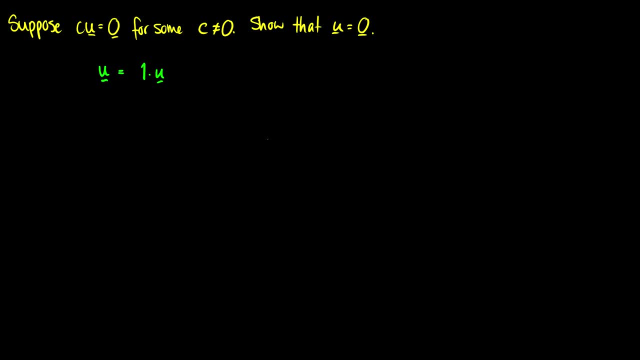 So maybe that'd be a little bit easier, because now we have this one here that we can work with. and what's nice about one? Well, what's nice about one is that in algebra, if we have a number, say c, and we multiply it by its inverse, one times c, then we get one back. So we can change this one. 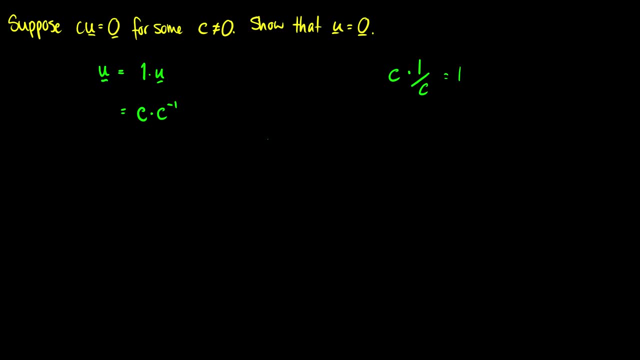 to be c times c inverse times u. Okay, so. so that's a really nice property of the number one is that 1 is equal to c times u times C inverse, And because C is non-zero, we can do this Okay. so now the next step. 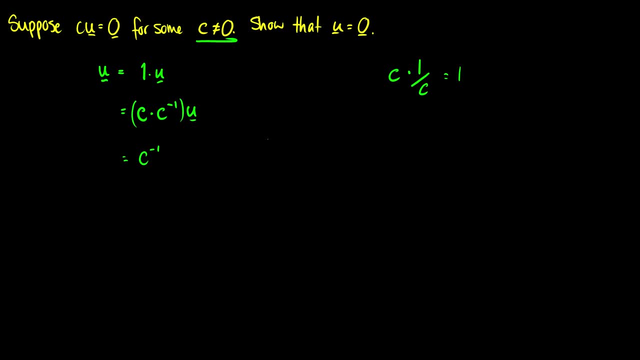 we should flip these around for commutativity. So we're going to have C1 times C times the vector U, and then we should group up this C times U together. So why do we want to group up this C times U? Well, we do that because we suppose that C times U is equal to the zero vector. 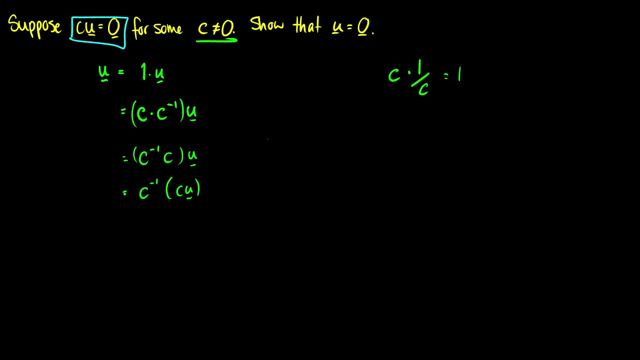 We're just trying to prove that U is equal to zero. So we know C times U is equal to the zero vector. Therefore, we know that this is going to be equivalent to the inverse of C times the zero vector. So what's the nice thing about the zero vector? Well, we know anything times the zero. 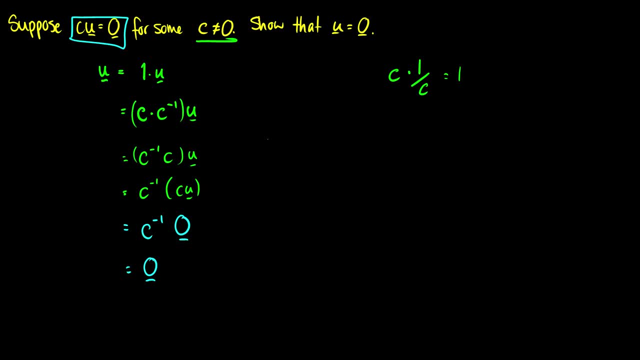 vector is just going to be the zero vector. Therefore, we have shown that U is equal to the zero vector. Okay, so those are two proofs with subspaces. If you have any questions, please leave them in the comments below. Pretty much all of the practice videos for